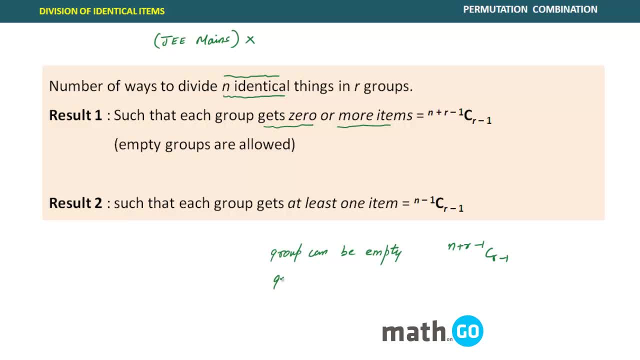 right, They could be empty. also, When you say that groups cannot be empty, that means each should have at least one. they should not be empty. then the answer will become n minus 1, c, r minus 1.. Just remember this. this is just a formula. I'll just show you how you'd apply. 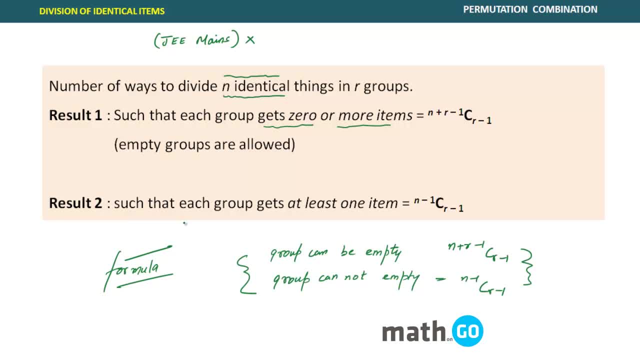 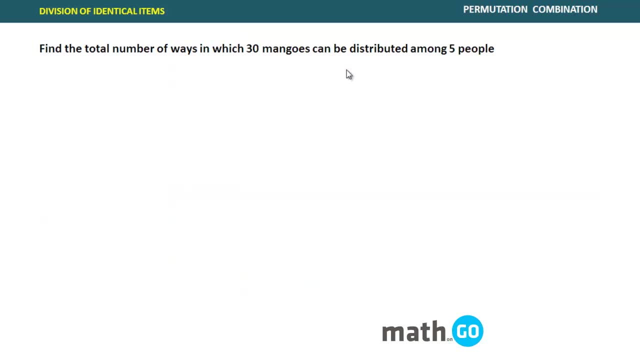 this formula. So this is just a formula. I'll just show you how you'd apply this formula- this in the problem, so you will get comfortable. Okay, minded that these formulas are valid when you are dividing n identical items, not distinct items. Now let's see the question. It says: find: 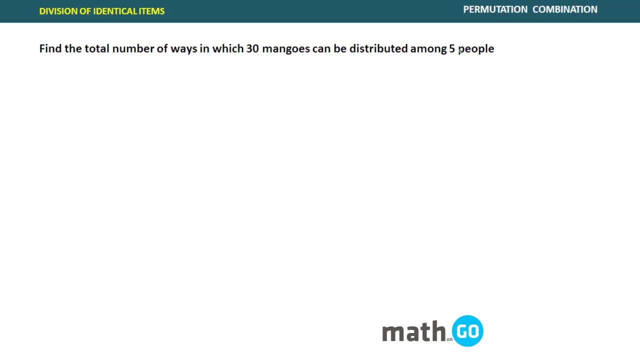 the number of ways in which 30 mangoes can be distributed among five people. So all the mangoes are identical. So first of all, just understand that mangoes are identical. No need to. you know, given this in the exam. mangoes are identical to. n is equal to 30. Right, And how many people has? 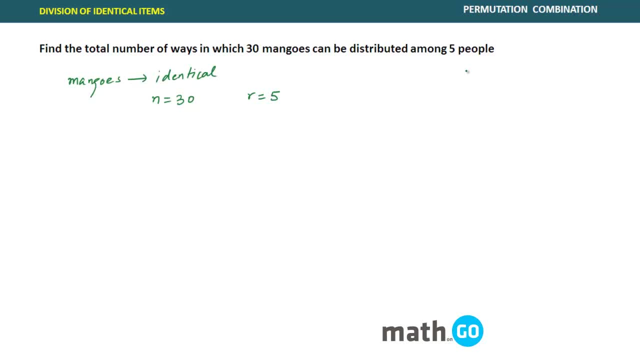 to be given five, any other condition that given to you. So it could be that all the 30 mangoes are given to person one only. This is true, right, There are five people. So it is not sure it is not given that. 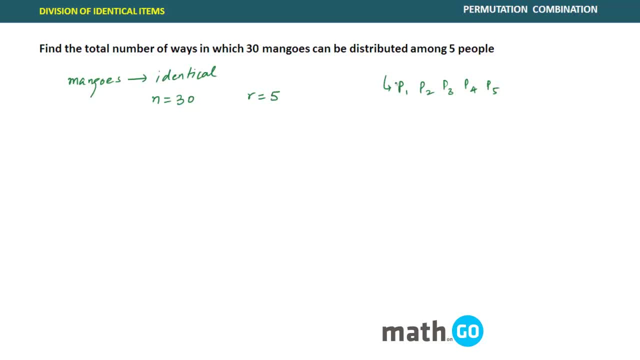 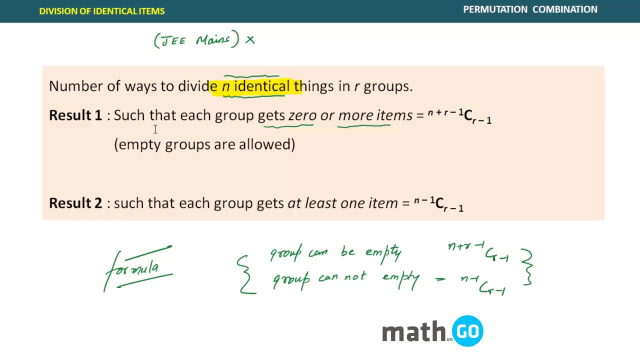 how many is the minimum value that should be given to each one of them? So I can give all the 32 person one also. So the answer that you are going to use is which one? just see to this, the first one or the second one? Second one is for at least one to each item or each group. No, 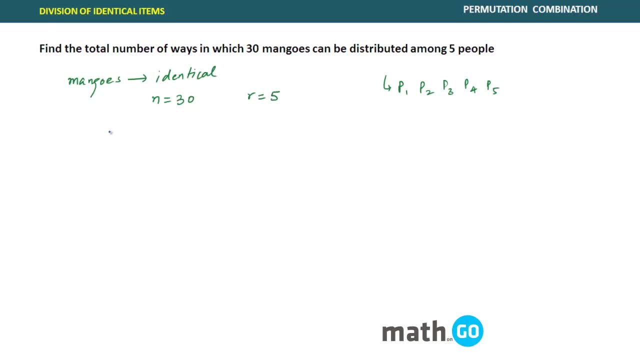 it is not given here, So we'll use what? Yes, So the formula that we are going to use is n plus r minus one, C r minus one. So how do we apply this is 30? Plus five minus one C. Yes, five minus one. 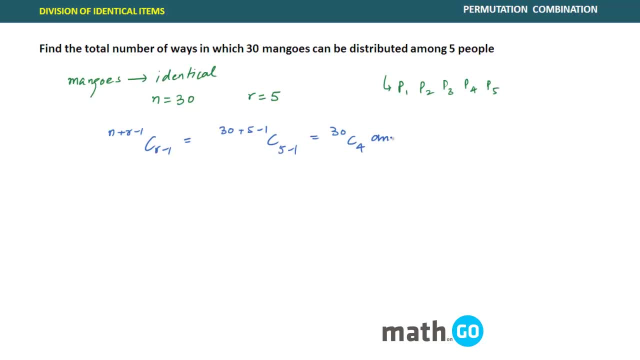 This is 30 c four. This is the answer we are looking for, And there's always all these kinds of questions. Let's do more of this right. This is something very beautiful, And they are asked in some various forms. So, for example, this is the category of questions which are asked. 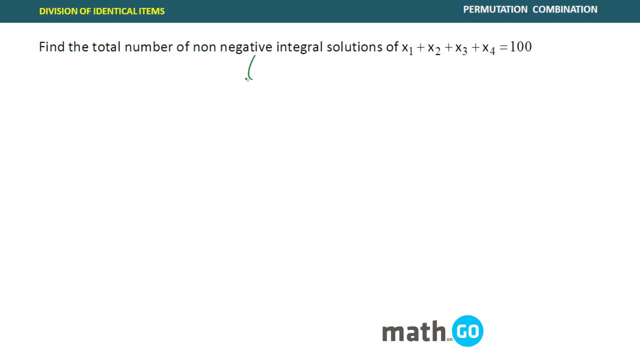 Find the total number of non negative integral solution. So what do you mean by non negative? First of all, non negative means 0123.. This is the meaning of non negative right. So that means whole numbers we are talking about. So never start non negative from one zero is a non negative. 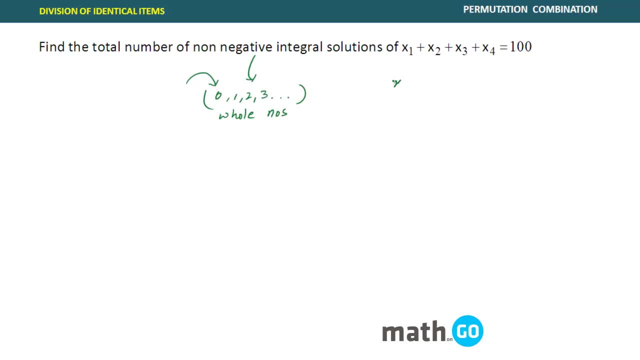 number, right, So we'll start from zero. So you want values of x one, x two, x three and x four which belong to your whole numbers, right? Or let's say I write here, which belong to whole numbers, And also they satisfy that their sum is nothing but. 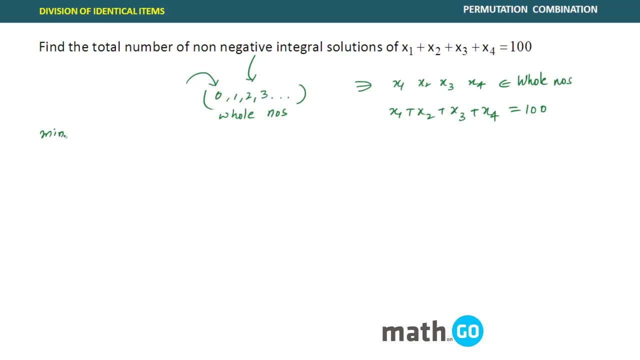 100.. Right, What is the minimum value that x one can take? min of x one is zero. That means you're getting it now. Yes, yes, yes, you are. you people are getting it, I hope. So it is actually equivalent. 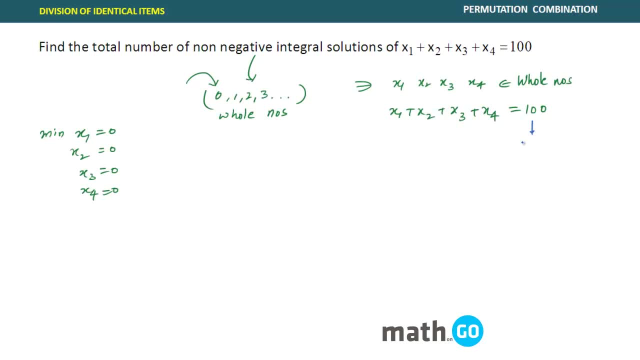 to saying that 100, 100 is what when you get 100? 100 is something when one is written 100 times And all ones are identical. One are identical. So that means how many identical items are there with you? They are 100 identical items, then only you will get 100. So for this, 100 items are to be. 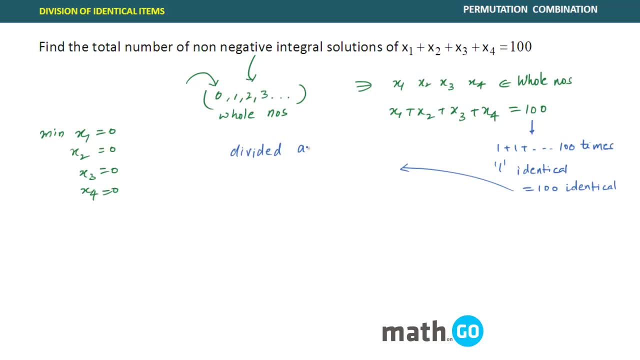 divided among how many people? divided among four boxes or four groups? Right Groups are x one, x two, x three And your x four. we need to divide them in these four groups. got it such that each group can get zero or more. Here is the condition. What do you will use again n plus r minus one. see r minus one, That said. 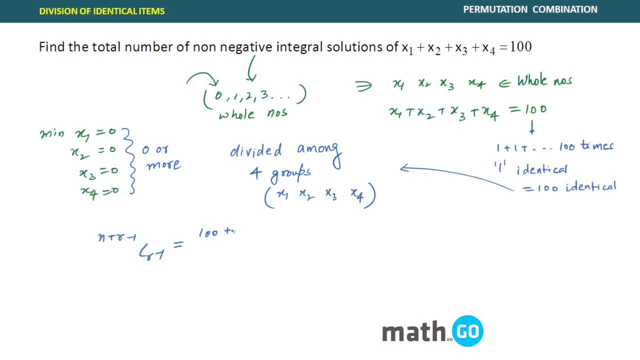 can you see this simple this problem was. it looks like a very intimidating problem at the first, but this is nothing. a very simple problem. So this actually is hundred three c three. So this is the answer you're looking for over, and if I had to change, 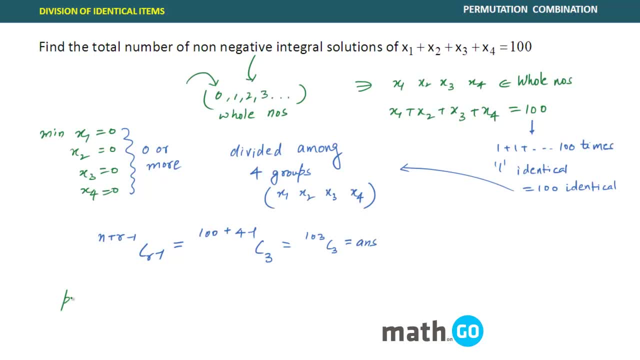 a simple, very simple stuff in this question. if I say find positive integral solutions, positive integral, so what the answer would be then? a positive integral. the value of x1, x2, x3, x4 will now belong to natural number. natural number start from. yes, they start from one right. so that means now. 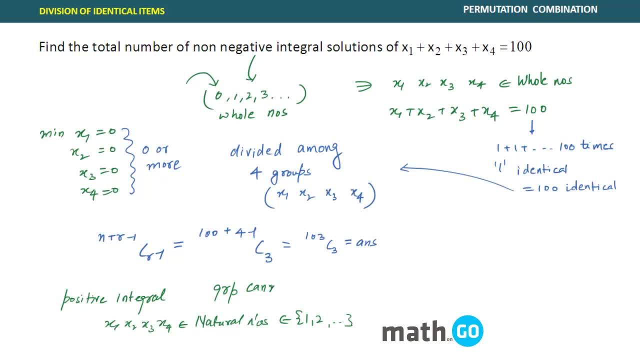 the group cannot be. group cannot be empty because at least one item should be there. so if group cannot be empty, what the formula would be? n-1, c, r-1, for the answer to this problem will then become 99, c3. then this would be the answer. I hope this is getting clear to you. 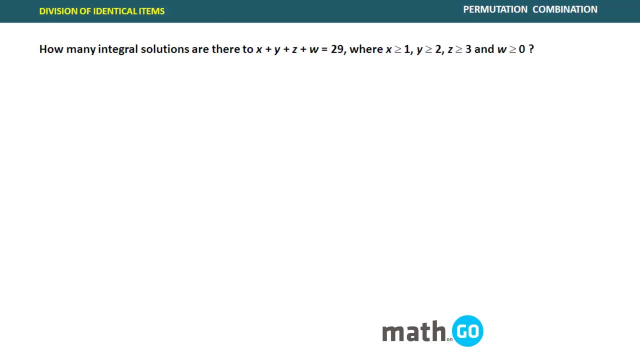 so now the again the same problem, though we call them. if you want to get hold of how, what is this we are solving? this is called integral equation method, right? so we are doing this basic of integral equation method, though it is much more than this. so it is: x plus y plus z plus w is equal to 29. 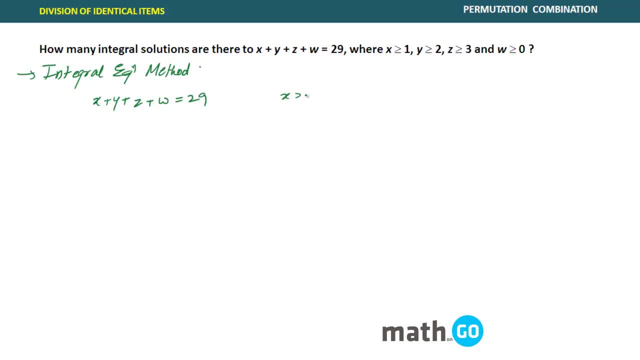 right, and it is also given that x is greater than 1, y is greater than 2, z is greater than 3 and w is greater than equal to 0. right now, we want to divide 29 into four groups, such that this is the condition which is given to you. 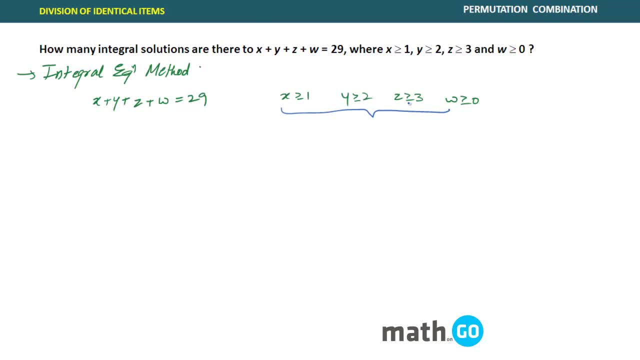 but the conditions are very varied. it is not that each group should be empty or more. what you should do this, try and do something of this sort. but everybody group- what do you mean by this is W group can take zero or more. this is the meaning of this particular statement. 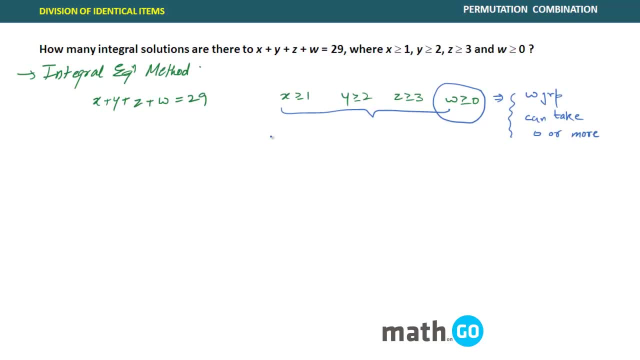 and we want each group to have the same category. so what we'll use? so let G will replace x by capital X plus one. right, so this becomes capital X is nearly ten approached Sonali capital. why plus two? we are doing this just to form zero capital z plus three, greater than zero. this gives you: 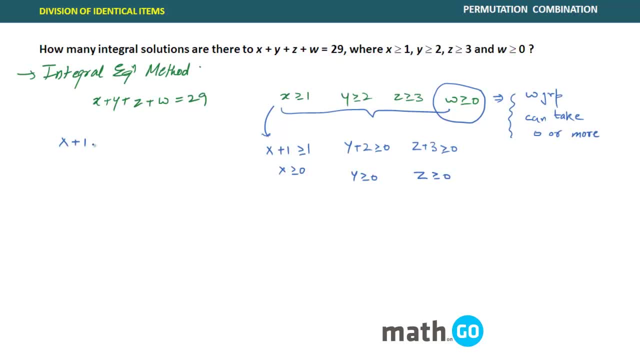 capital z is zero, and if you do the substitution here it becomes c. this right, and for w we do not require anything, right. so now this question simplifies to this particular concept, right, where we have to subtract six. so either you solve this or you solve this, does not matter. so now the question is 23 into four groups, right, where each can get. 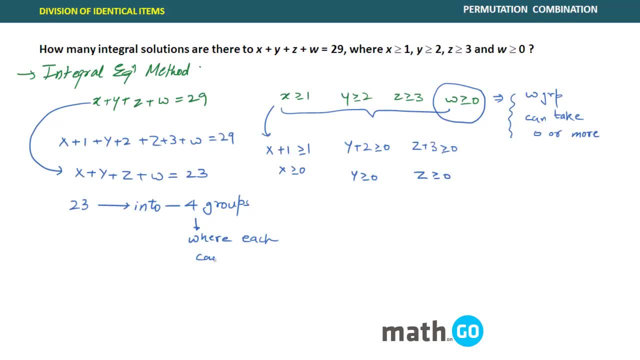 zero or more, where each can take zero or more. got it zero or more? this is what is meant by it, because now, if you see the condition here, here, here and w is already greater than zero. so now we know the answer. the answer is n plus r minus one, c r minus one. this is how we are.